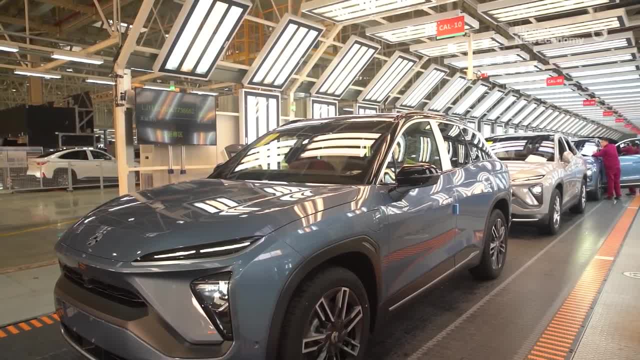 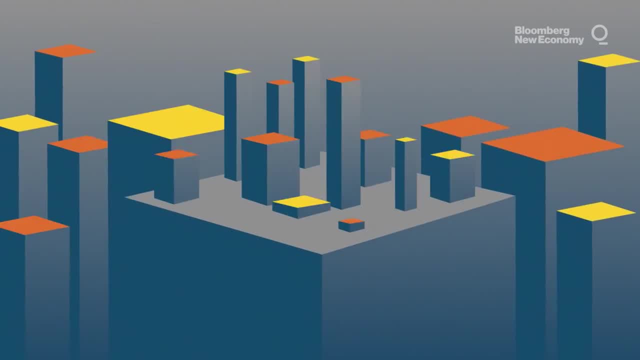 all the way down to your EVs and your battery packs. How the West deals with that. they're going to have to be a bit creative. What China plans to accomplish by 2030 could determine the shape of the global energy system of the future. 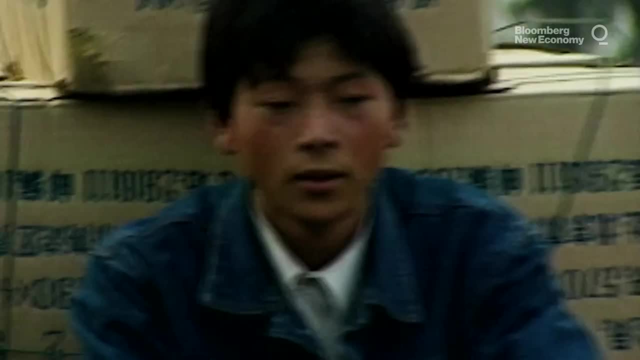 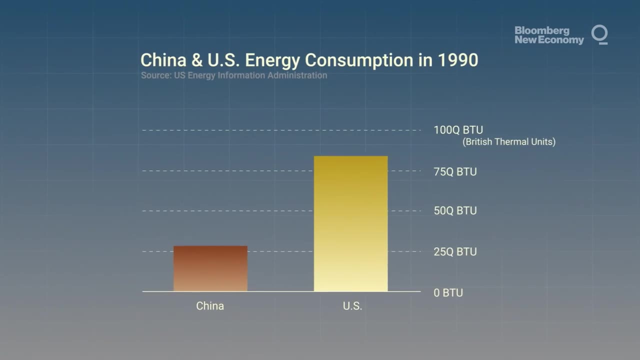 At the end of the last century, China was on the cusp of an economic revolution. In 1990, its GDP was only 6% that of the US And its energy use was only 34%. The economic reforms of the 80s and 90s. 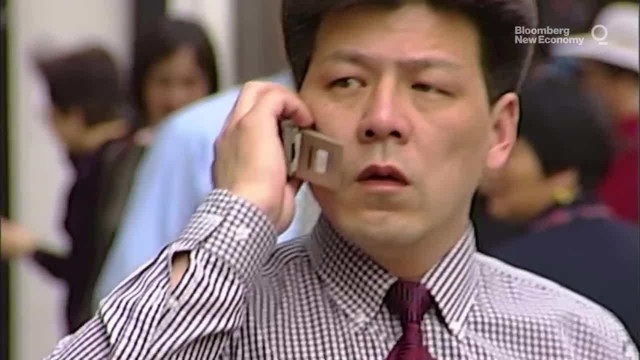 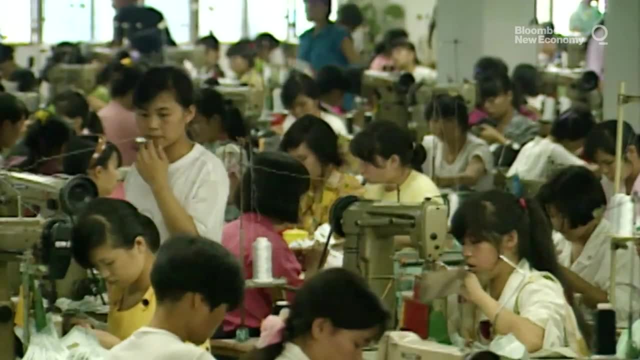 started the process of privatising industry and opening up to trade with the rest of the world By the time it joined the World Trade Organisation in 2001,. China was well on its way to becoming the world's factory, with booming energy needs to match. 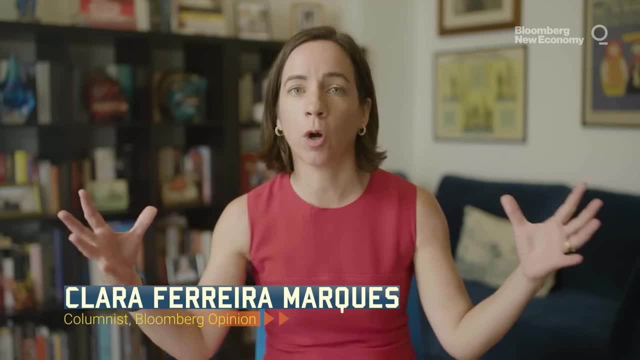 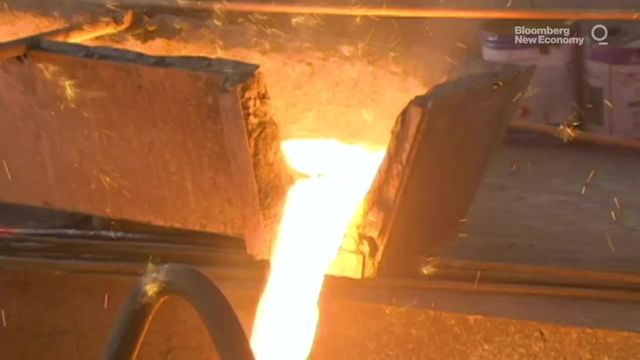 The history of it is really dramatic. I think just the condensation. Really China is doing industrial revolution a hundred years after that. all of that in a very concentrated period of time. So what we saw is obviously dramatic change in terms of energy consumption. 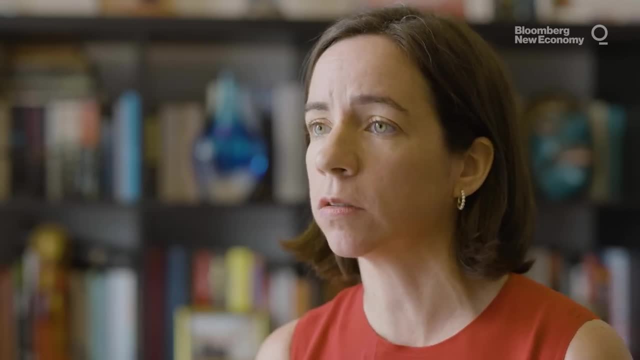 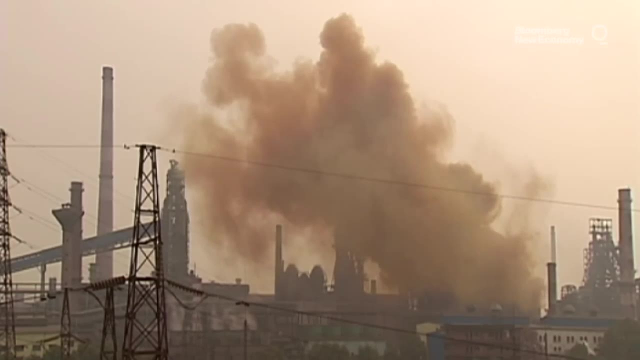 and there were power crunches in the early years where really the system was still trying to cope. dramatic addition of coal-fired plants in particular. to deal with that From a climate perspective, the position was: well, you had your turn, now it's our turn. 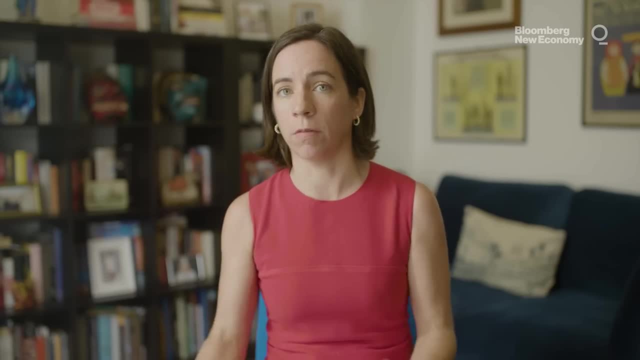 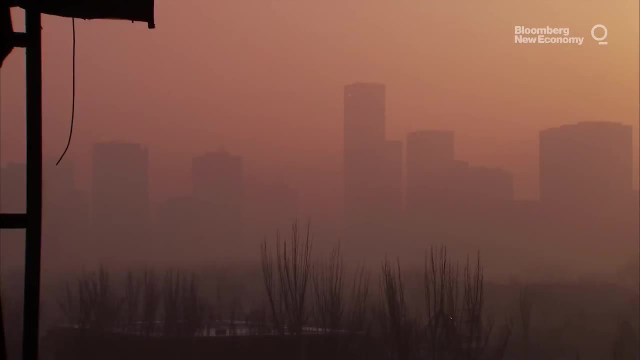 When you were growing you as the West, there was no question of what carbon was doing. You did whatever you wanted. now it's our turn. That really changed in 2008,, 2009,, and that coincides with an awareness of air pollution. 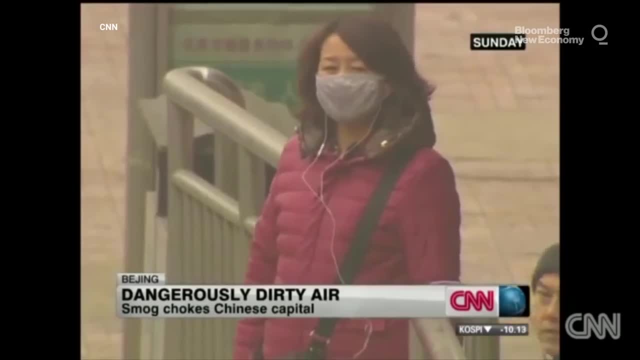 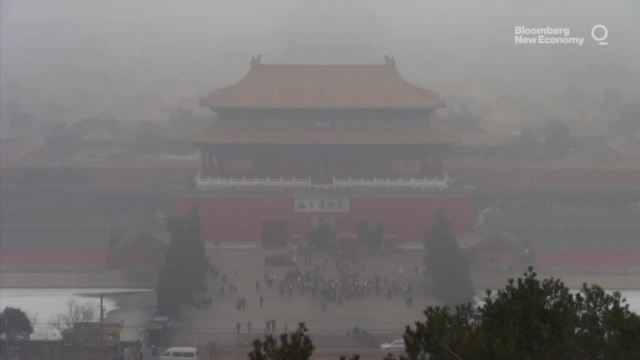 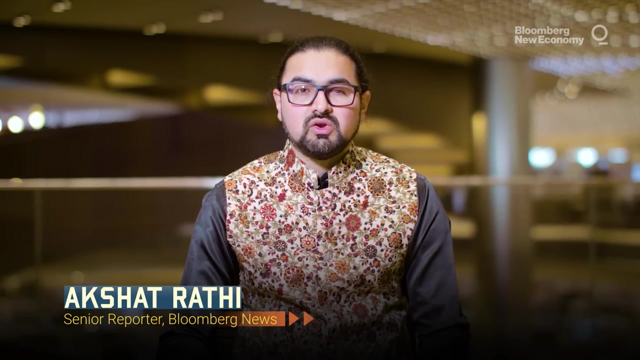 In Beijing, which is facing another smoggy day. some environmentalists say it is the worst air on record. Beijing was famously the most polluted city in the world for almost a decade. It also became very clear to its leadership that that kind of growth will be unsustainable. 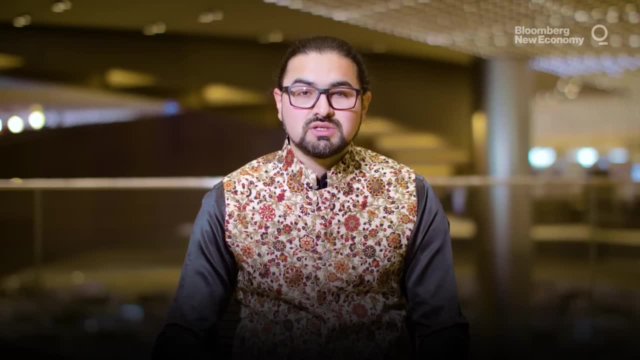 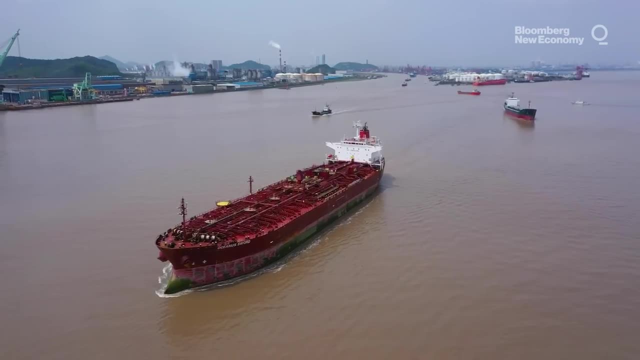 not just from a fact of putting out a lot of emissions, but from a fact that much of the fossil fuels consumed, for example, oil and natural gas, will have to be imported, And that's something China wanted to walk away from. So, starting about 2010,, 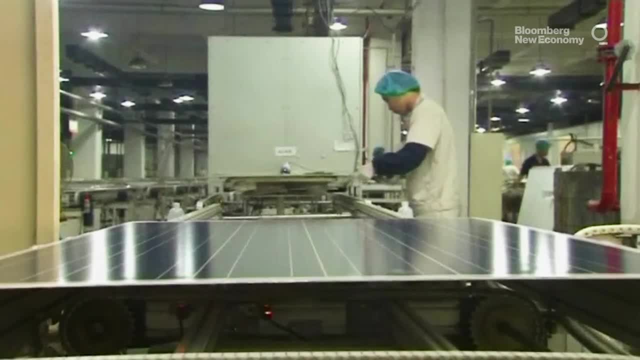 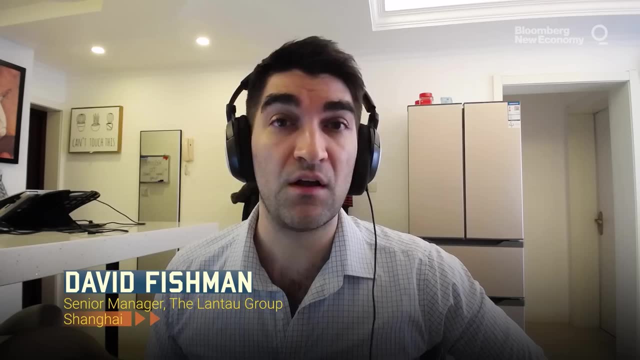 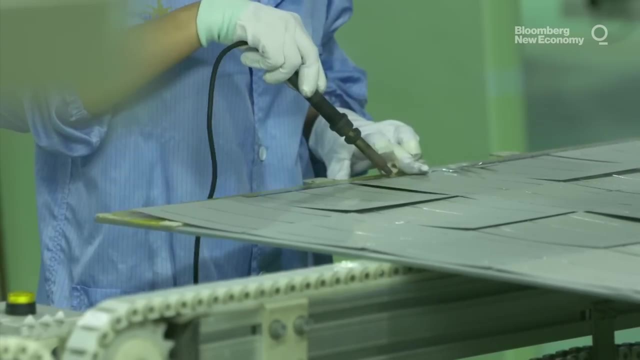 China committed to increase its deployment of renewables. China, like many other places in the world, was faced with initially very non-competitive on a cost basis economics for solar projects, for wind projects and being able to subsidize the manufacture of the key components. 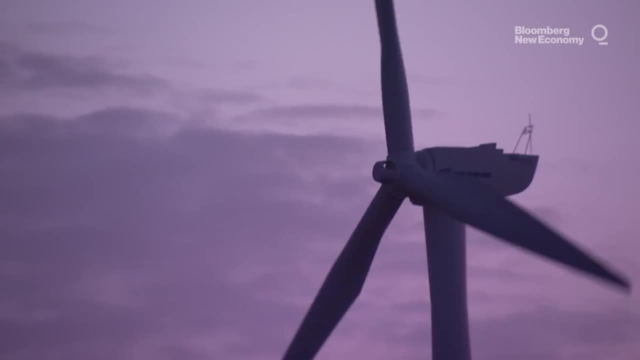 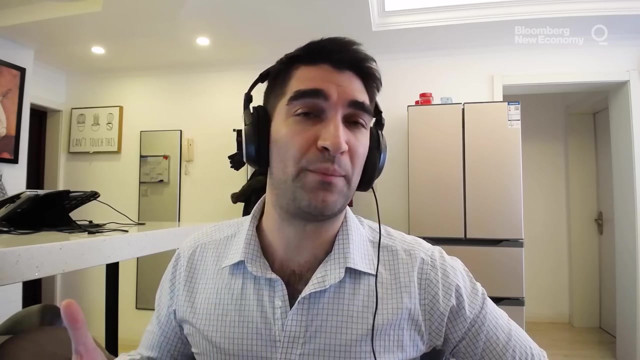 ensuring the power that they sell has an attractive rate. All of these things China has done very, very well. You push the market into existence and then you're able to pull back with some of the policy mandates because now it just makes good economic sense. 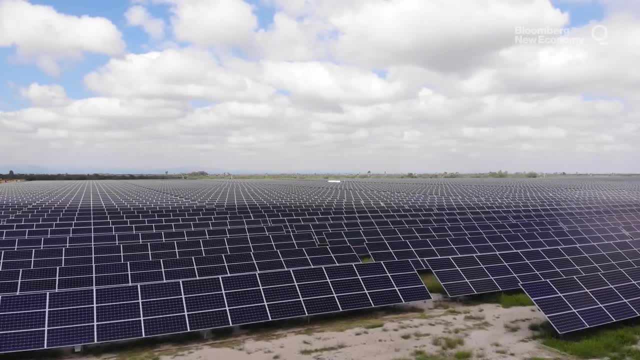 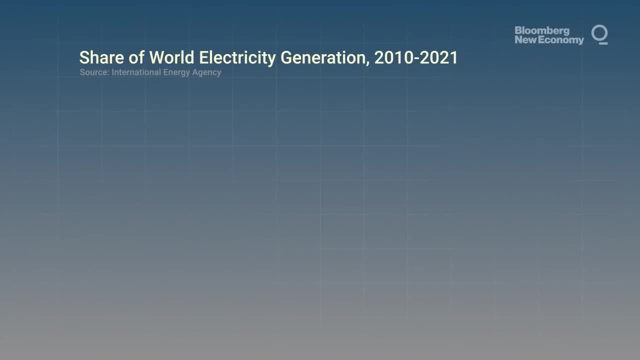 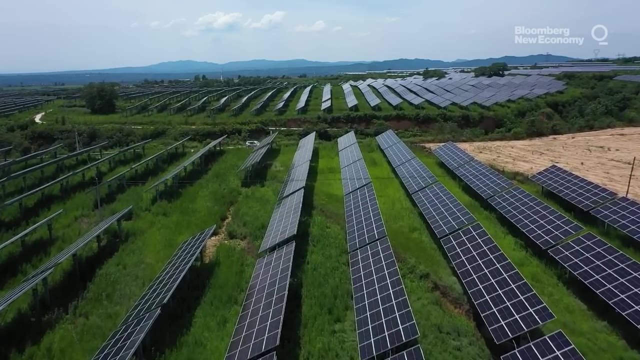 China's investments in renewables helped drive astonishing price drops across the industry, leading to record levels of new wind and solar installations all over the world in recent years. Last year, wind and solar generated more than 10% of the world's electricity. Still, renewables only make up a tiny fraction. 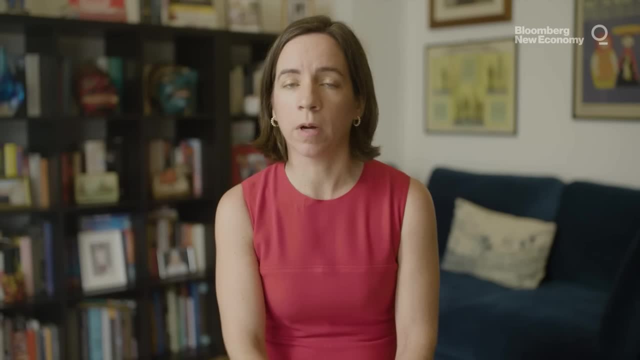 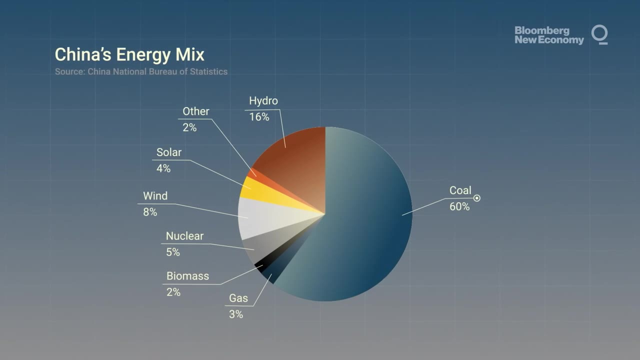 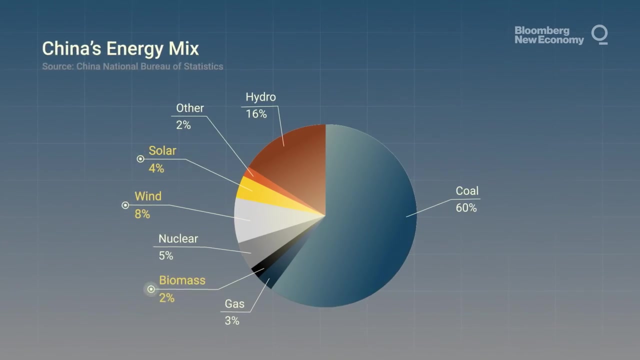 of China's energy mix today. China is overwhelmingly dependent on fossil fuels at the moment And within that, if you look at power generation, it's overwhelmingly coal- roughly 60% Wind, biomass, solar remain a much, much smaller fraction. 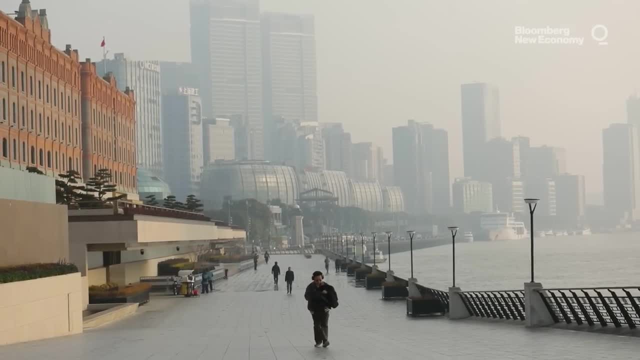 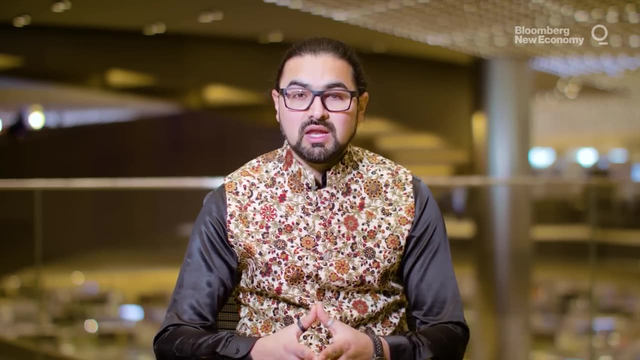 There was pressure building up on China for quite a few years that China needs to do something, It needs to do more to cut emissions, And that finally sort of came together in 2015 at the Paris Agreement, when China agreed to sign it alongside the US. 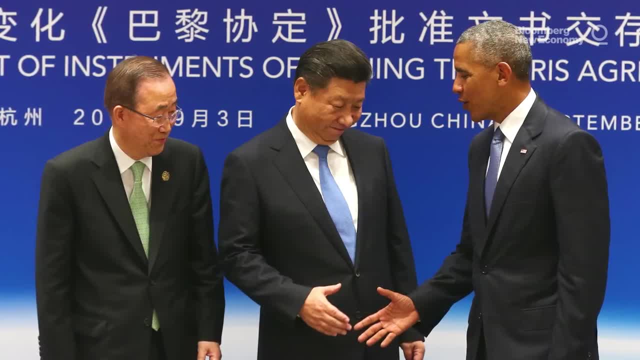 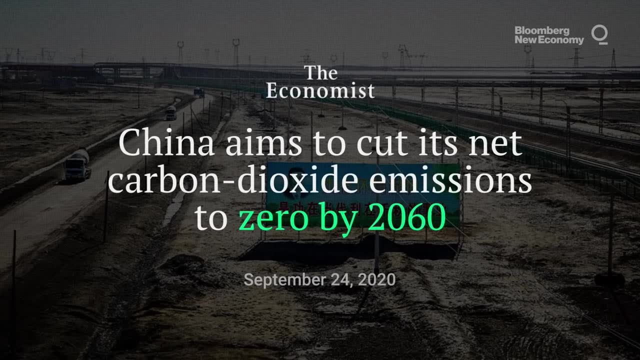 and pretty much every country on the planet. That bit of diplomacy was crucial to take China to the next stage, which is when, in 2020, it declared that it will set a net zero goal, And, in a way, it was a coup for China. 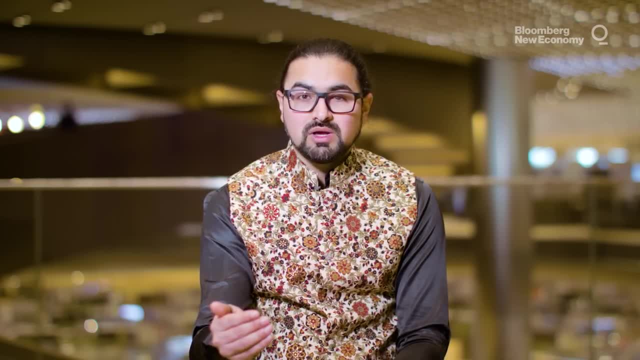 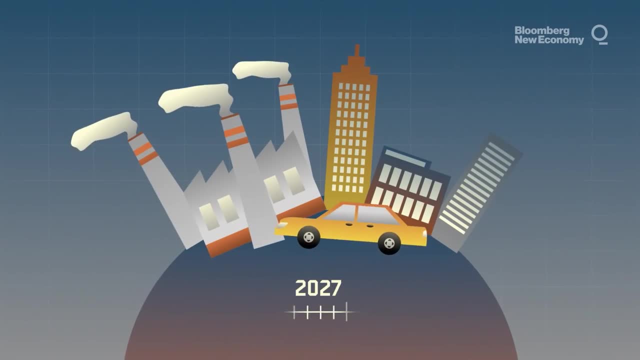 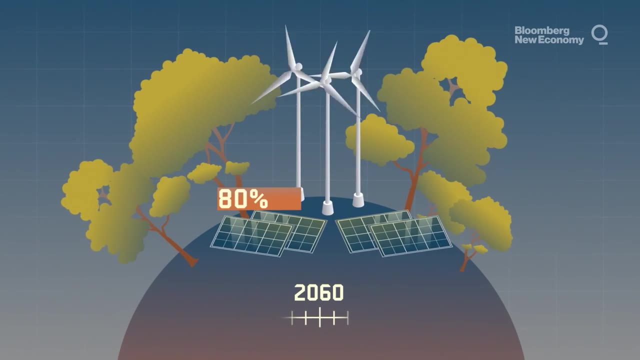 because it set that goal even before the US could have done so. China's decarbonization plan ramps up gradually, with fossil fuel emissions increasing for a few years before peaking in 2030.. From there, they've given themselves another three decades to get to net zero. 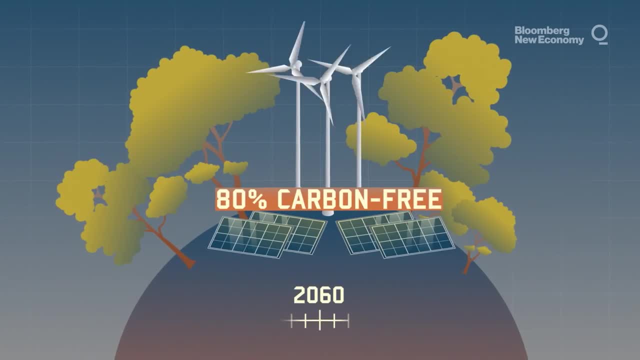 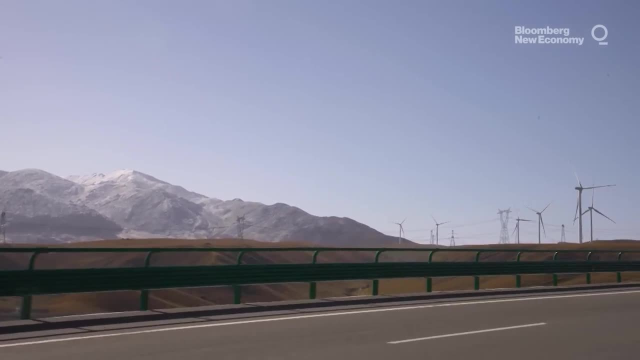 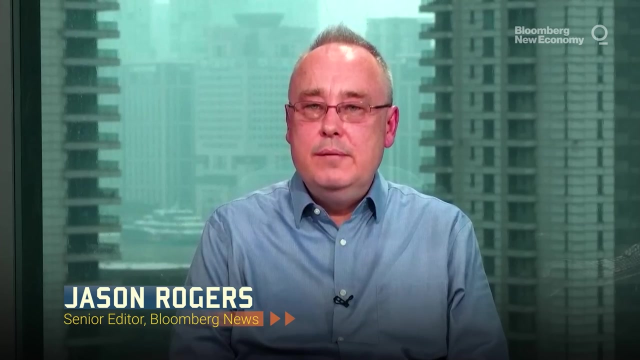 with 80% of energy coming from carbon-free sources by 2060.. Getting there will be a massive undertaking, and it starts with renewable megaprojects on a scale seen nowhere else on Earth So late in 2021, we took a reporting trip to Qinghai in western China. 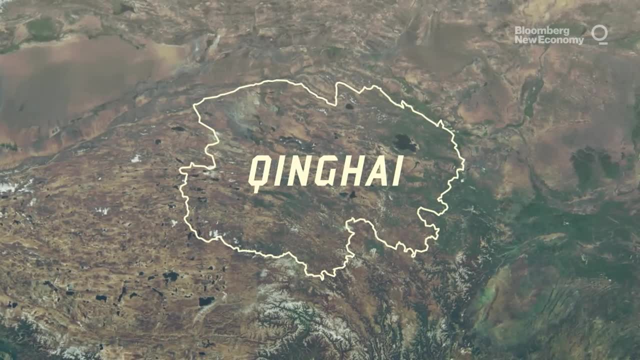 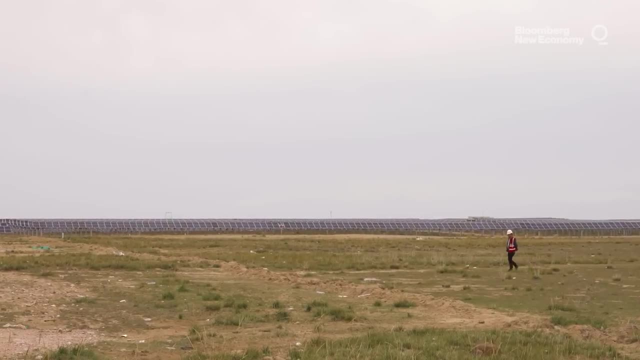 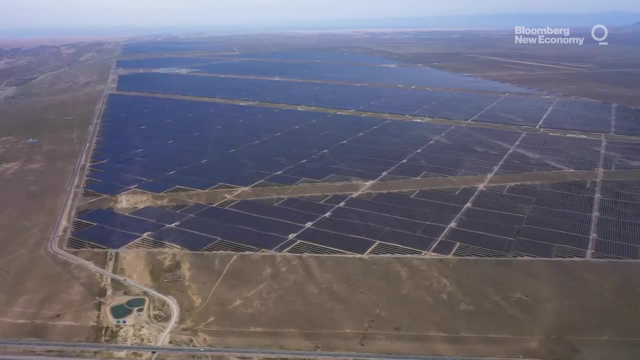 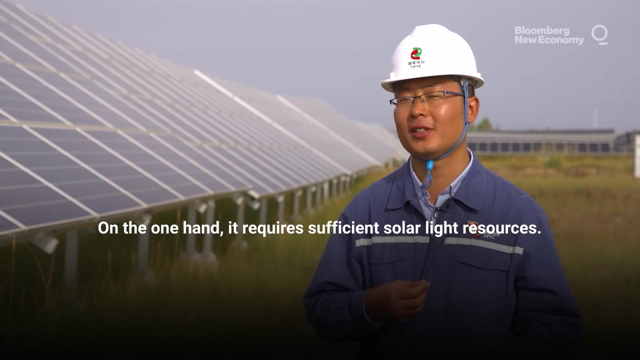 It's quite windswept. it's a very sunny part of the world, very low population density. We went to a facility that was spread out over 600 square kilometers, about the size of Singapore. It's got a lot of solar energy and solar energy resources. 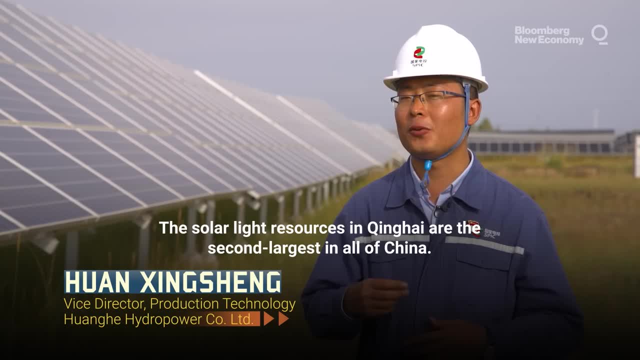 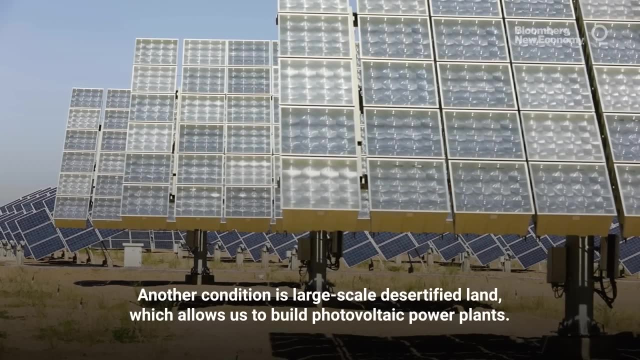 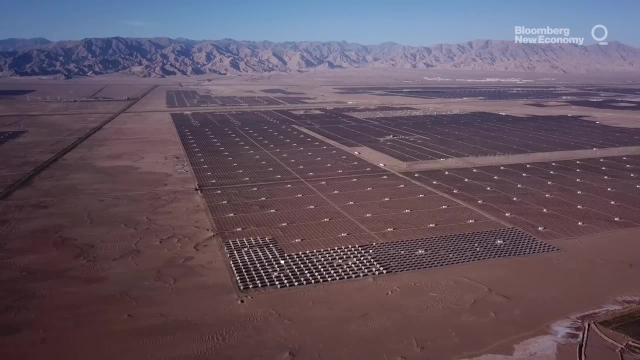 China ranks second in terms of solar energy resources in Qinghai. Another condition is that we have a large desert-like land. We can build this power station with the original land, But these two resources are inevitable In that facility. you know they have a hydro dam. 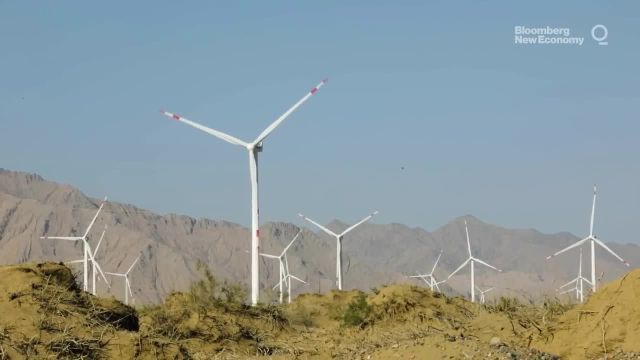 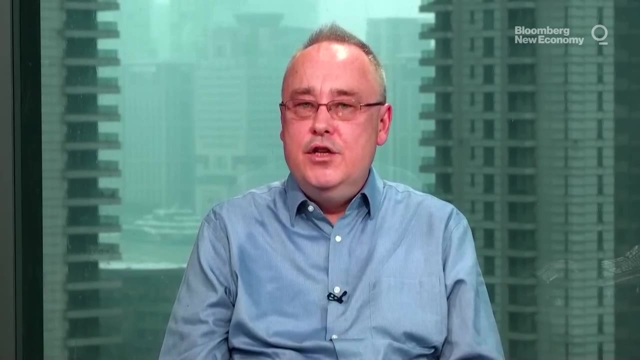 They've got a massive solar build-up and they're adding wind installations as well. If all of that is up and running, it's going to be producing nearly 20 gigawatts of energy. It's enough to cover the power needs at any given time for Israel, for example. 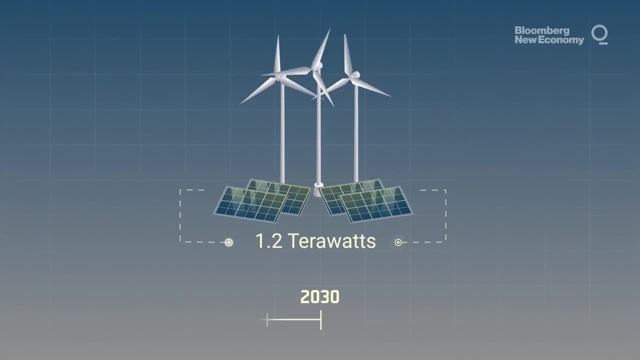 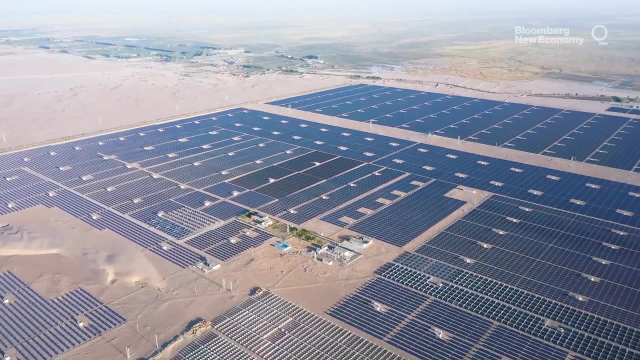 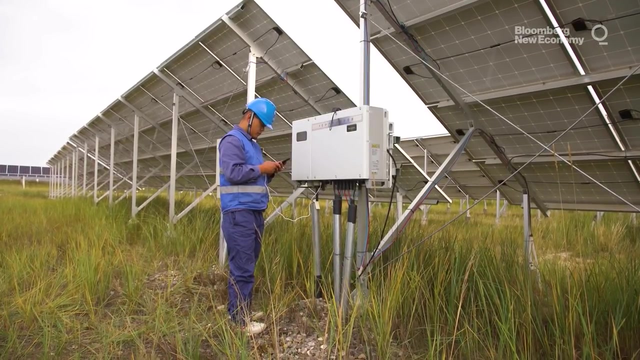 By 2030, China plans to scale up to 1.2 terawatts of wind and solar capacity- enough to meet all of the US's electricity needs today. But it's not enough just to generate that power. Getting the power where it needs to go is a megaproject in itself. 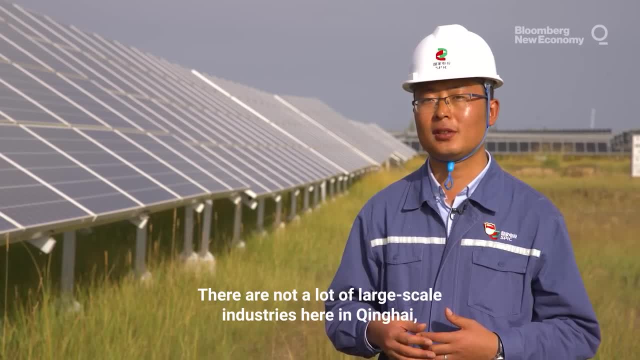 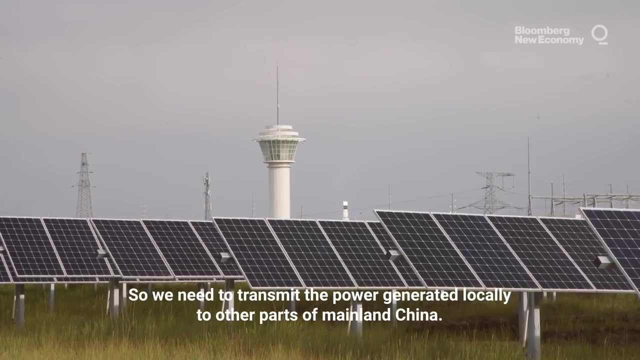 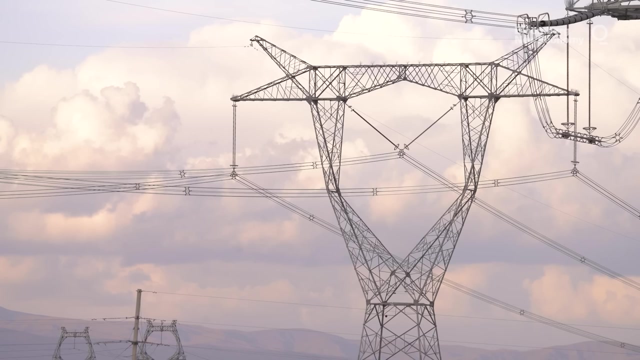 There's not a lot of large-scale heat industry in Qinghai And we don't need that much electricity, So we need to transport the electricity we produce locally to China In order to ship all that electricity. China has basically built this huge network of ultra-high voltage power lines. 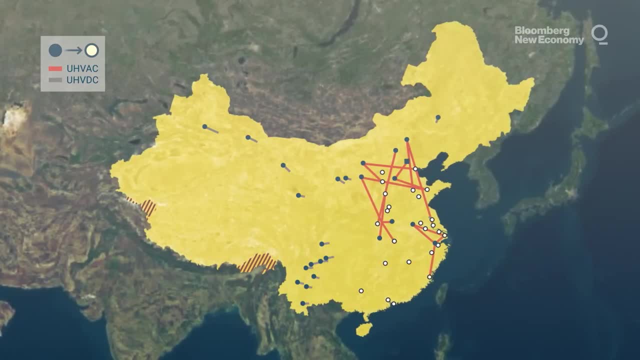 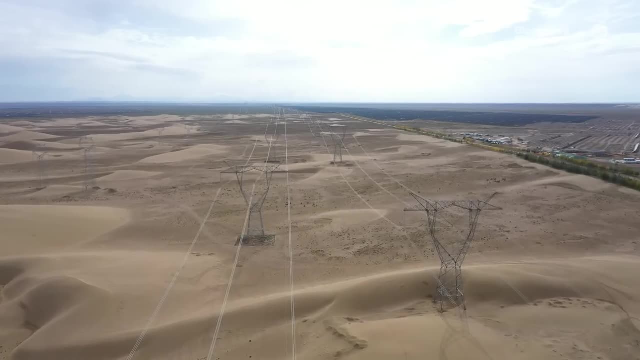 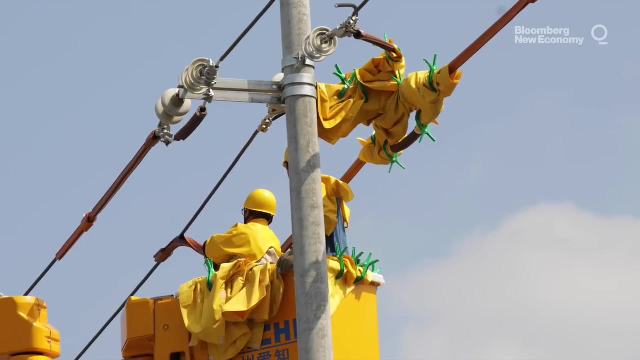 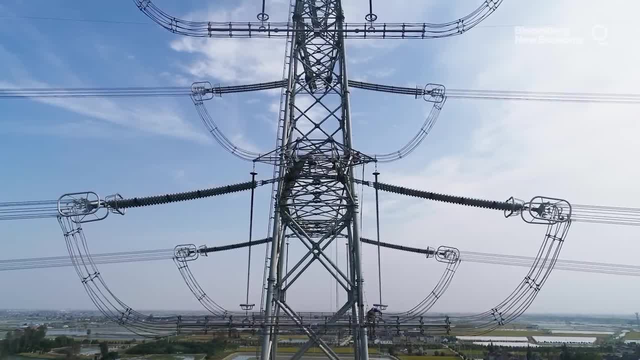 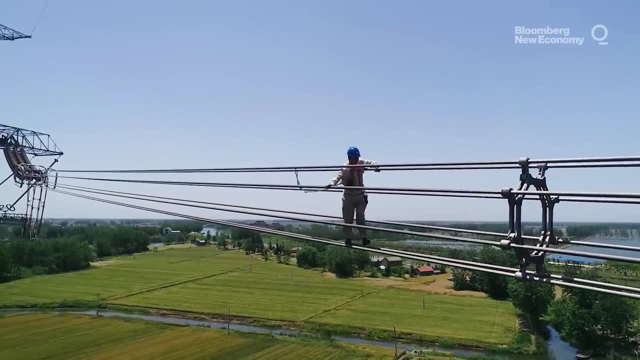 hence the need for these specialised direct current lines. What they do is they reduce the wastage that may happen on the way to transport this electricity. There are only two countries in the world where these cables are operating: China and Brazil. Brazil has two of those cables. 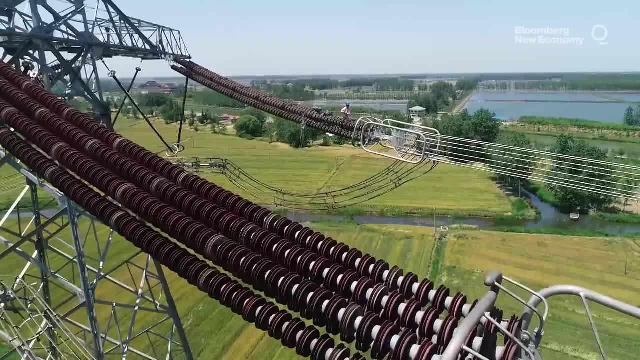 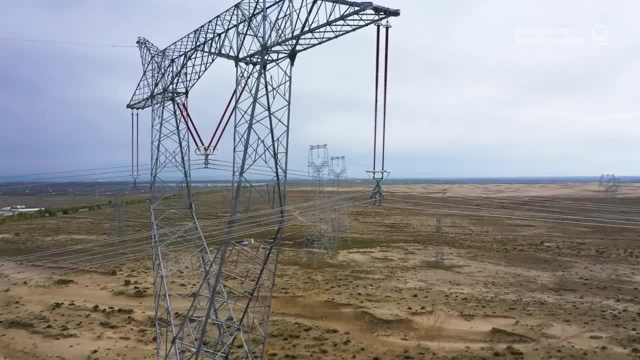 Brazil has two of those cables. China has 25.. By far and away, China is absolutely the leader on this, And the amount of money that you're talking about- I mean it's hundreds of billions of dollars that they're going to be spending on this in coming decades. 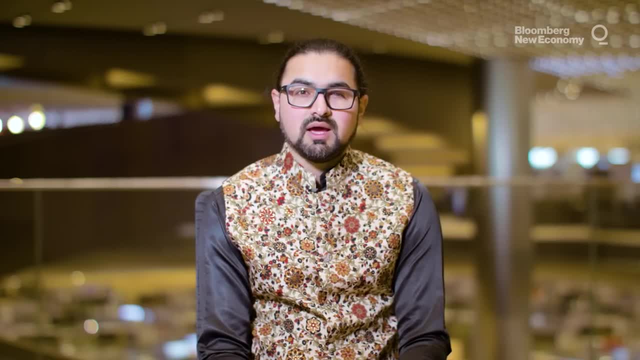 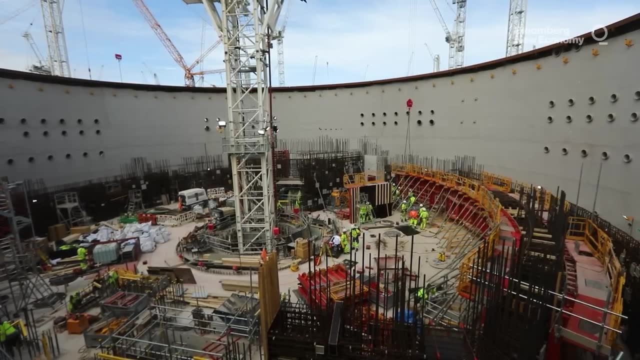 As China goes towards a net zero goal, its leadership has recognised that there is no way China can meet those goals without having what's called firm clean power. The idea of firm clean power is that you're able to generate carbon-free electricity when you want it. 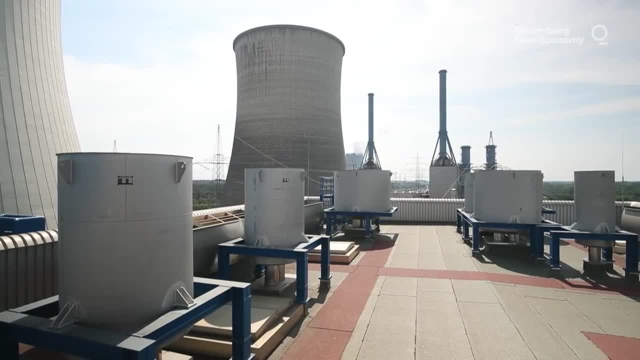 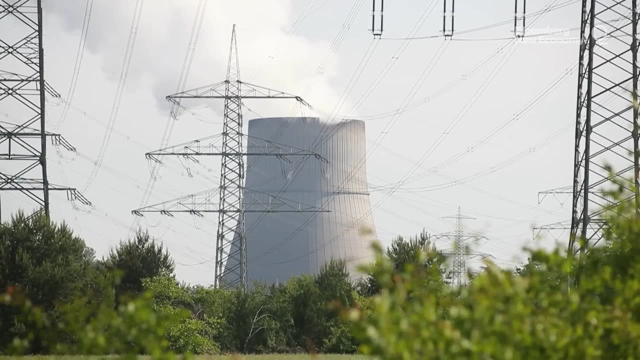 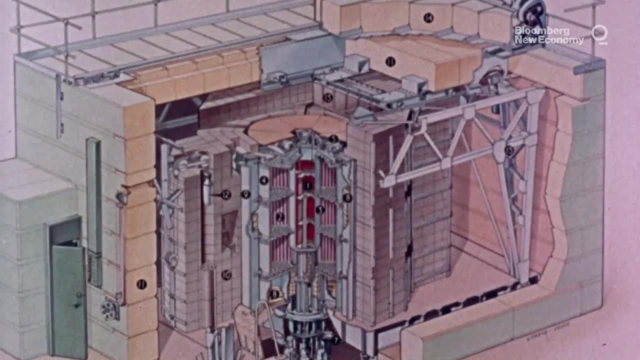 rather than relying on when the sun shines or the wind blows, Nuclear power satisfies those conditions quite well. In most countries the nuclear industry is struggling, facing huge upfront costs, regulatory hurdles and negative public opinion. Still, it is a carbon-free source of reliable power. 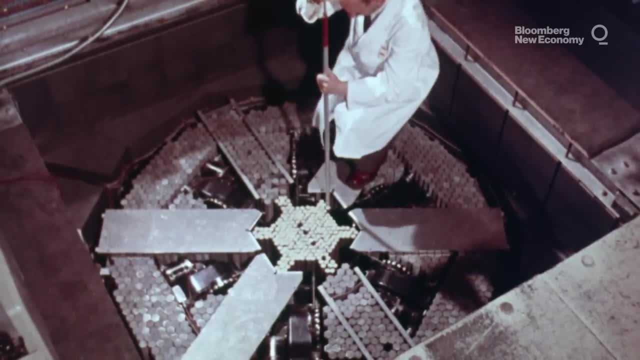 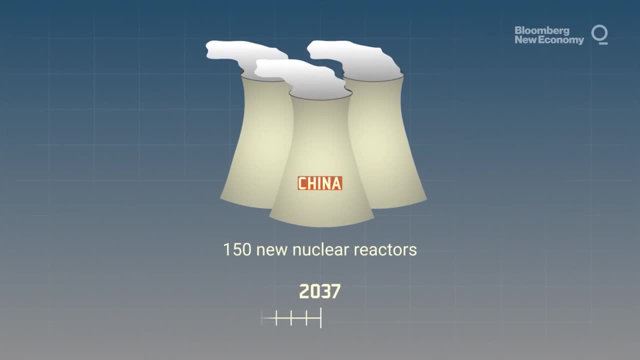 and many environmental advocates see it as a key to the green transition, as does China's leadership. China plans to build 150 new reactors in the next 15 years, which is more than what the entire world has built in the last 35 years. Nuclear isn't seen as controversial in China, or at least we don't know if it is. It's not clear whether China's own population supports it or opposes it, because they're not allowed to protest and show their opposition to a certain technology. 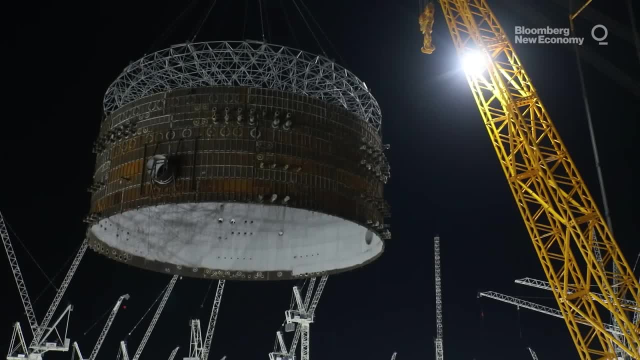 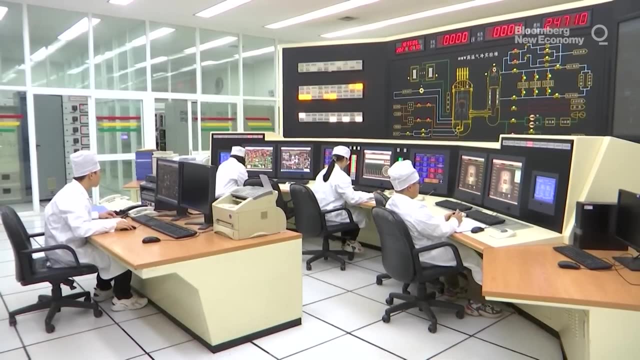 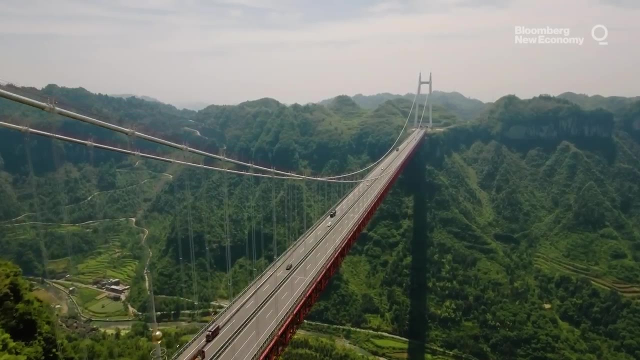 That still leaves the difficult economics of nuclear, the high upfront cost of building new reactors. Here too, China may have unique advantages. One thing that we all know China really excels at doing is building huge infrastructure quickly After decades of building bridges and skyscrapers and high-speed rail and ultra-high voltage lines. like every supermassive industrial project that China has built, that know-how goes into also building nuclear power plants. When you build projects consistently on schedule and on budget, you actually get to realize the benefits that were imagined back when the project was being planned. 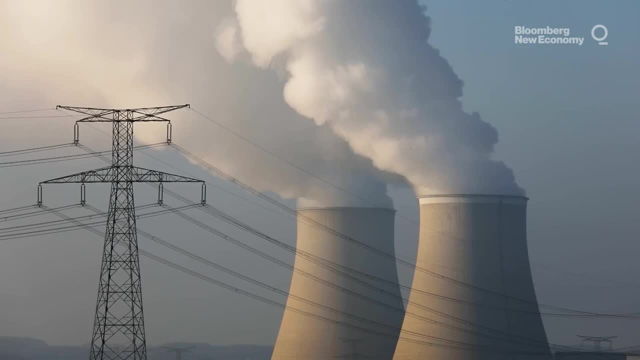 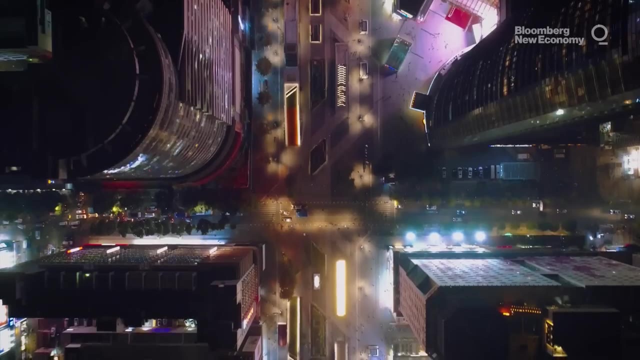 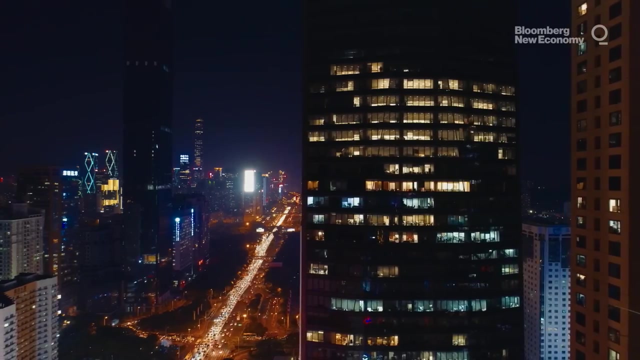 like stable, low-cost electricity, at a certain rate, at a certain production cost. China's efforts to decarbonize are likely to have many positive effects on its domestic energy supply, But that's not the only reason China has gone all-in on clean energy. 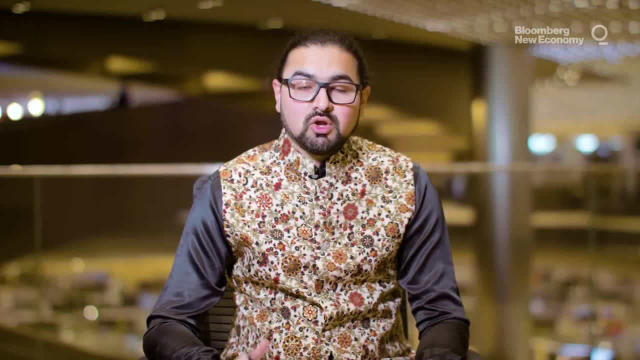 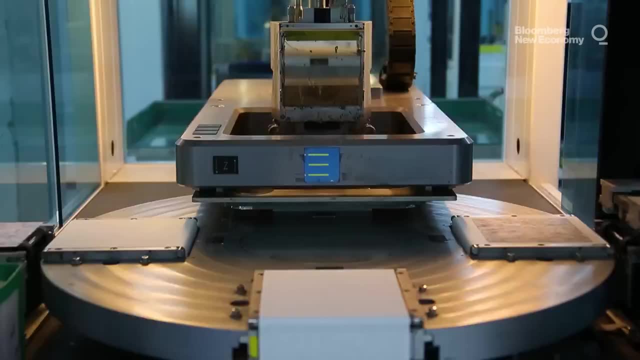 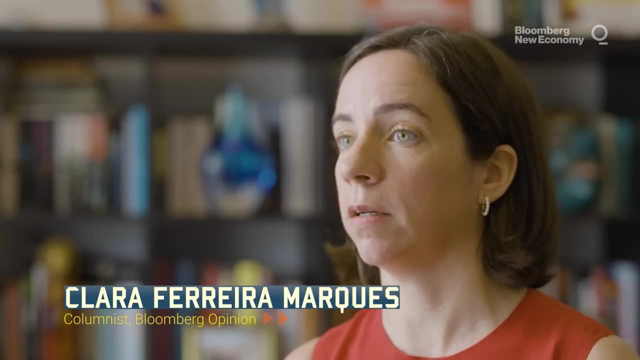 China certainly wants to meet a net-zero goal, but it also wants to be a country that is making a lot of money exporting the technologies that will clean up the energy system globally. China is incredibly important when we think about the supply chain for green technology in general. 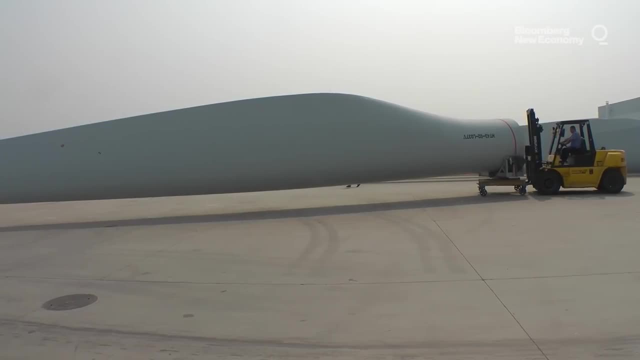 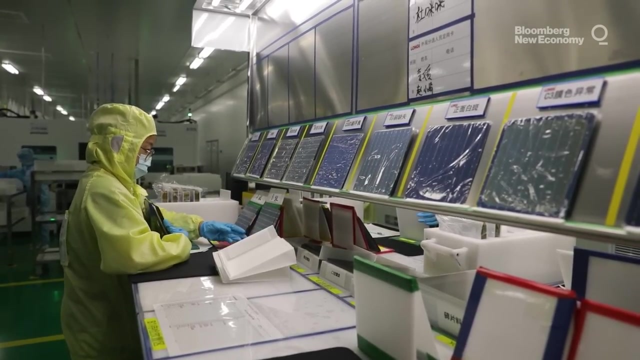 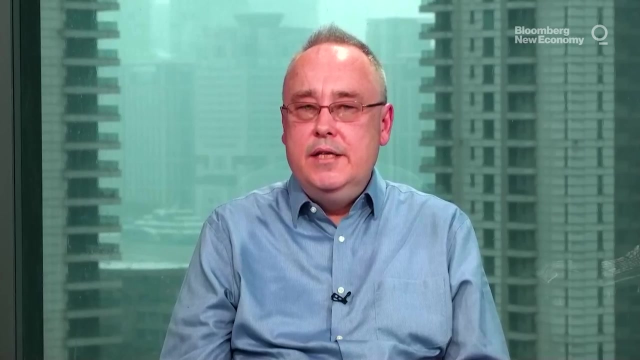 the green economy, whether that's solar panels or turbines or the elements that you need to process along the way, Incredibly significant. China basically accounts for something like 75 percent of the world's supply chain for solar. Anything that you're going to do in the States or in Europe, I mean at some. 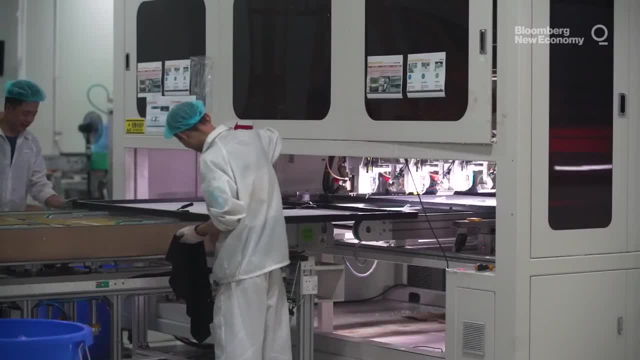 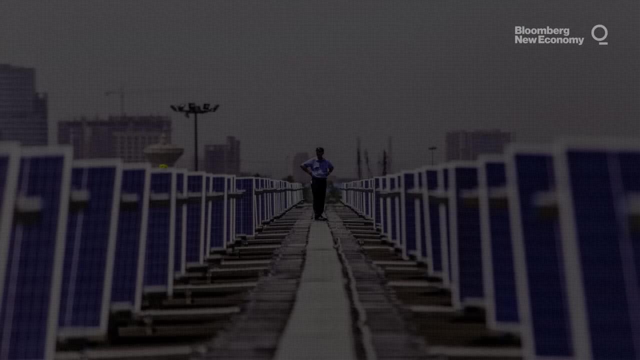 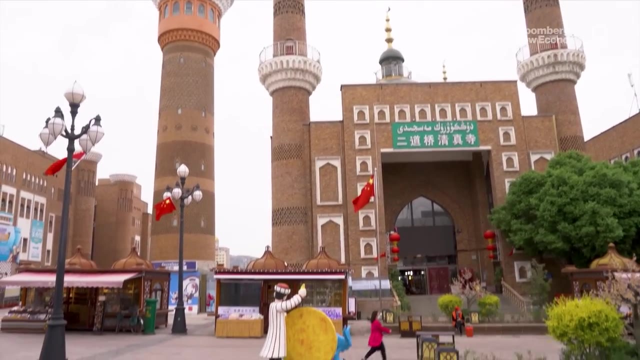 point, Chinese companies will have been involved in this. That dependence on China has lately been a source of strain. Last year, Covid-related production issues in China caused the price of solar panels to rise for the first time in decades, And some companies have pledged to take their business elsewhere. due to reports, 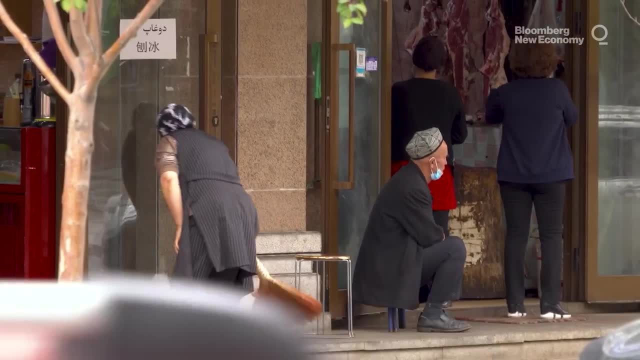 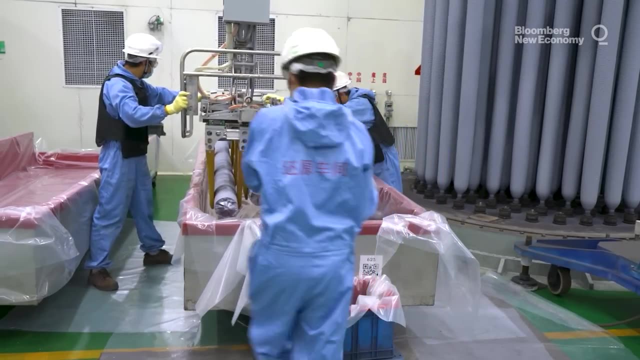 of human rights abuses in the majority Uyghur province of Xinjiang, which produces most of the world's polysilicon, a key material in the manufacturing of solar panels. Obviously, there have been accusations in the West that the Uyghurs are subject to forced 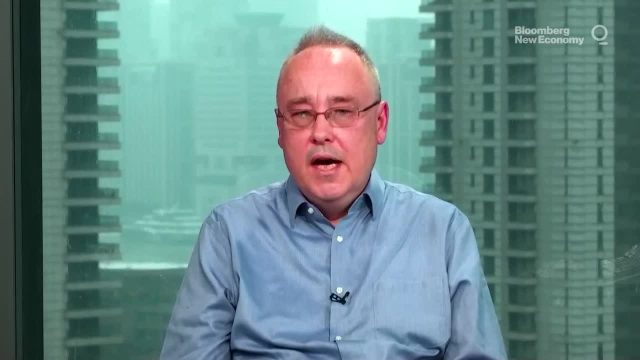 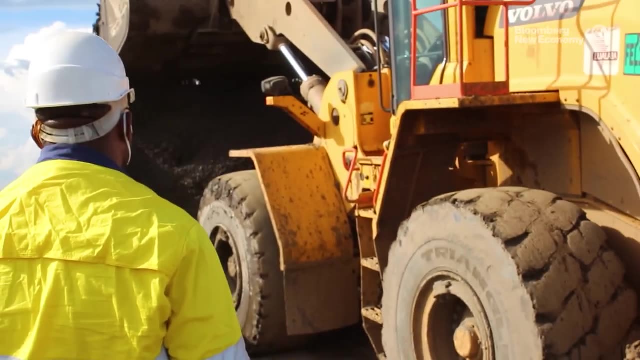 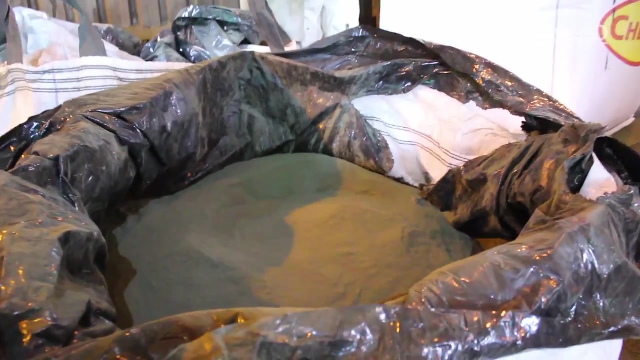 labour. The industry and the Chinese government have denied this. Some in the West are also concerned about China's dominance over the materials needed to make lithium-ion batteries. Cobalt, for example, is a scarce mineral produced mainly in the Democratic Republic of Congo, where China has bought. 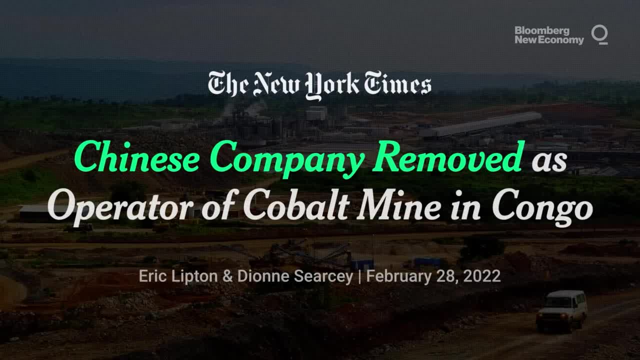 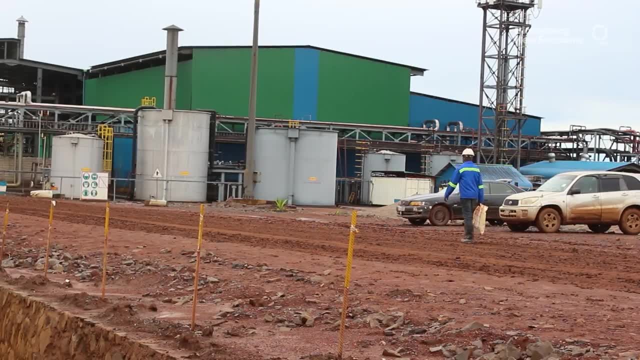 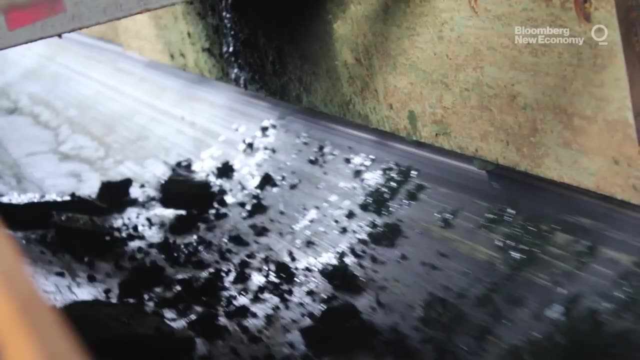 up most of the supply. The Congolese government has recently pushed back against those efforts, alleging poor working conditions and unpaid debts by a Chinese mining company. But the majority of cobalt-producing mines there are still, at least part Chinese-owned. Crucially, what China's done is it's also made the processing of these metals into the 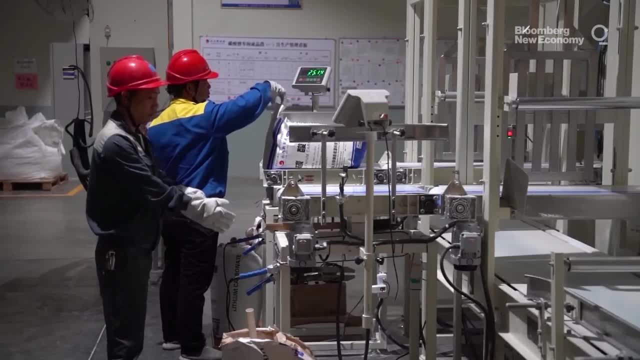 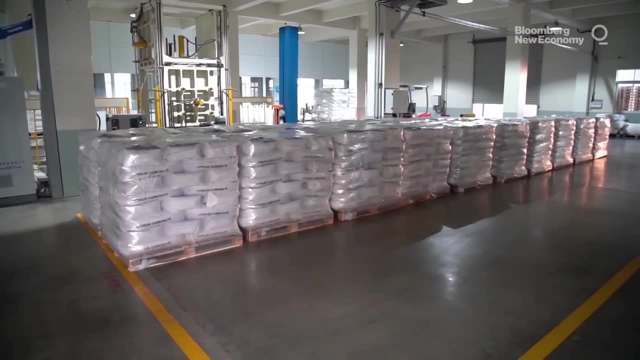 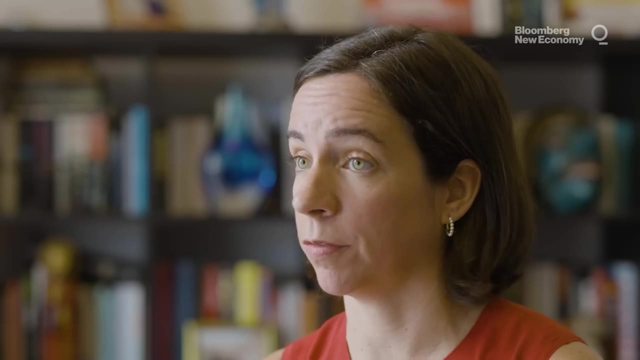 chemicals that eventually go into batteries, an almost monopoly. The processing capabilities of China outstrip those of all the rest of the world combined. I think any kind of excessive dependency is problematic, and energy dependency is no different. Think about Europe, Europe's dependency on Russia for gas. how problematic that has been. 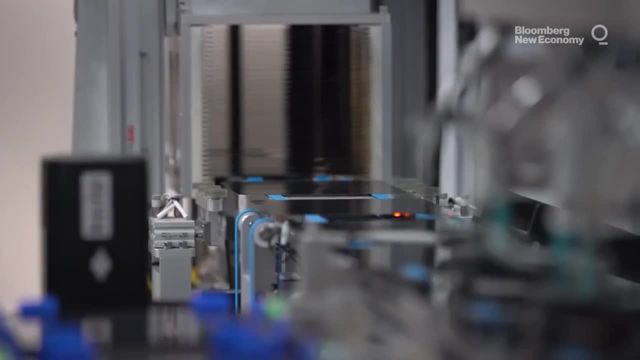 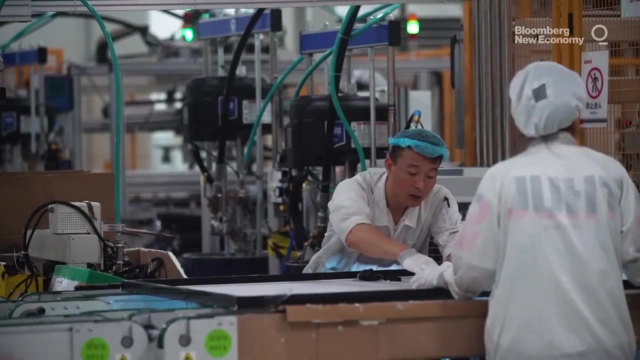 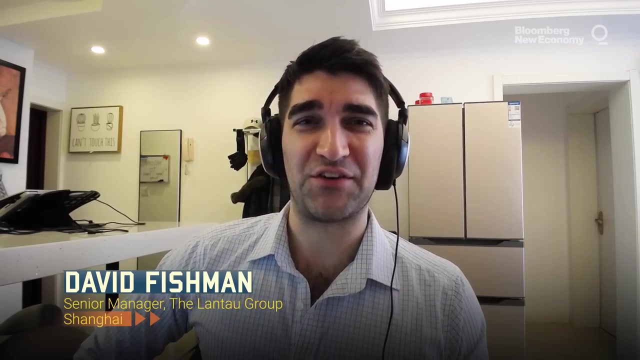 So if we're going to have that, the West as dependent on China for renewable energy, for green economy ingredients, it is not going to be a healthy situation. My instinct is that these things are not done for a nefarious purpose: right To dominate. 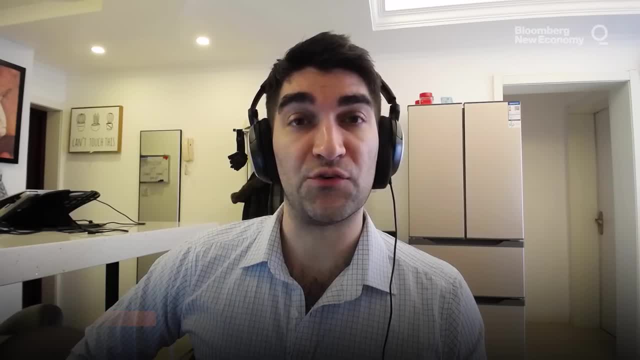 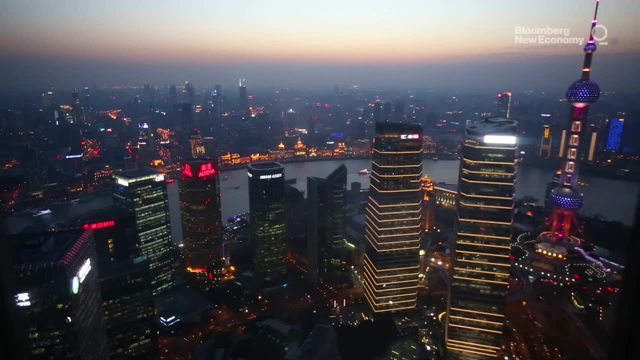 the supply chain in a way that is disadvantageous to another country. But you know that the primary consideration is what is good for China. I mean, remember, we're coming from a period of not so long ago- late 90s, early 2000s. when China had rolling blackouts all the time. China had a lot of blackouts all the time. I mean remember, we're coming from a period of not so long ago- late 90s, early 2000s- when China had rolling blackouts all the time. China had a lot of blackouts all the time. 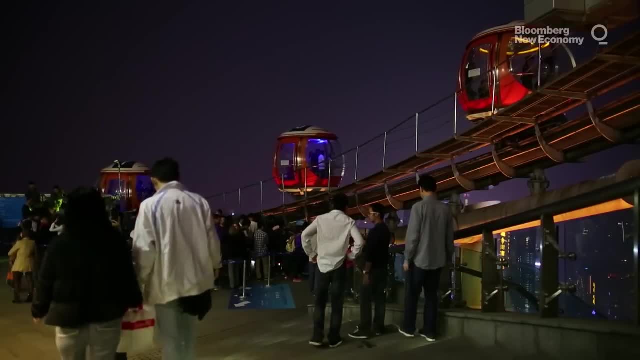 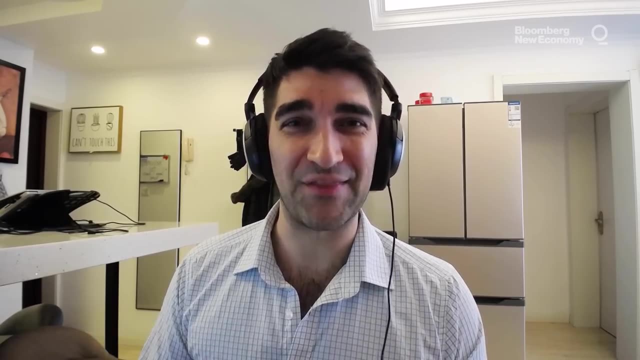 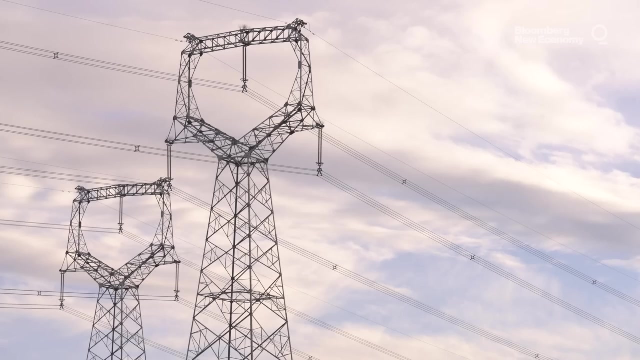 And we've got all this investment into making sure it can't happen again. From the way people talk about it here, they believe in the mission, and the mission is stable, secure energy for the Chinese people. Electricity rationing is being imposed in more than half of China's provinces. 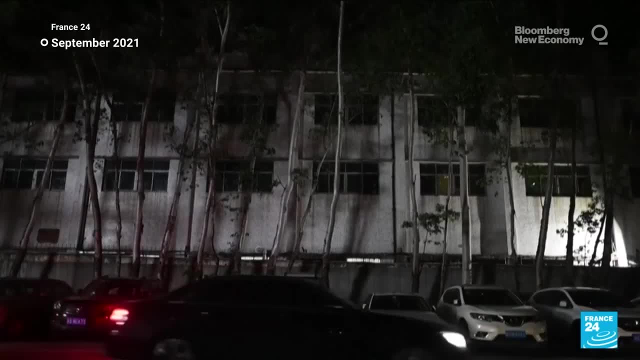 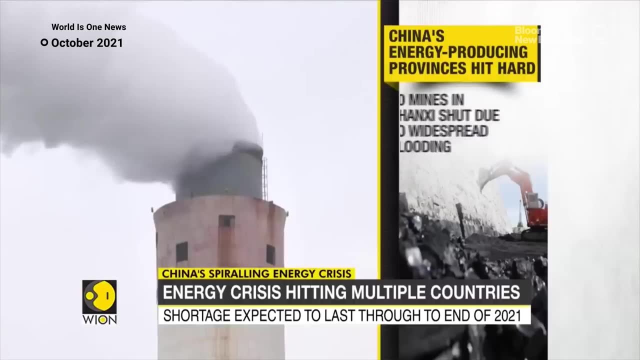 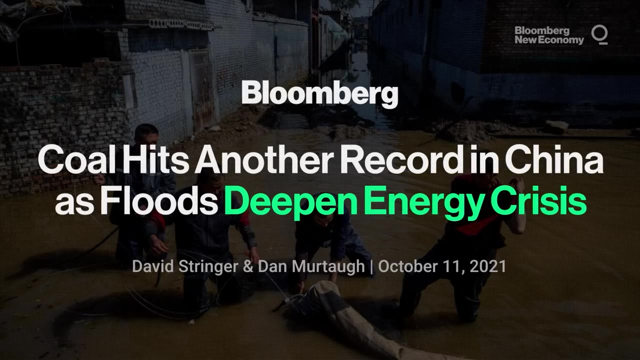 Power shortages are still ongoing. I think we've got a count of 20 provinces where there are electricity curbs. Recently, China has been having flashbacks to the bad old days of blackouts and power rationing. A sudden spike in the price of coal led to widespread power shortages —. 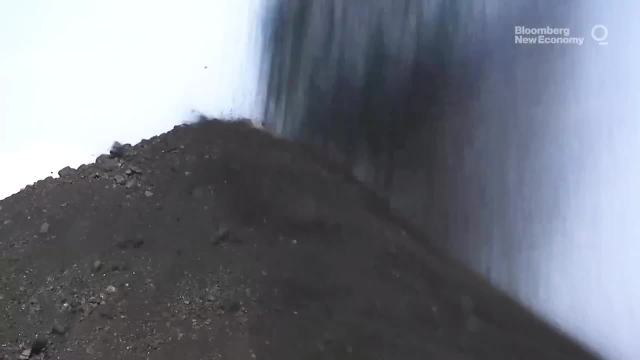 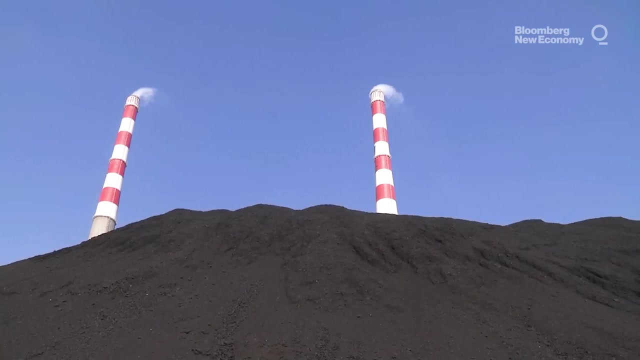 leaving the government little choice but to ration electricity and ramp up coal production. It's indicative of a major flaw in China's decarbonization plan. Even as they add world historic levels of renewables, they largely cancel out those gains with new fossil fuel additions. 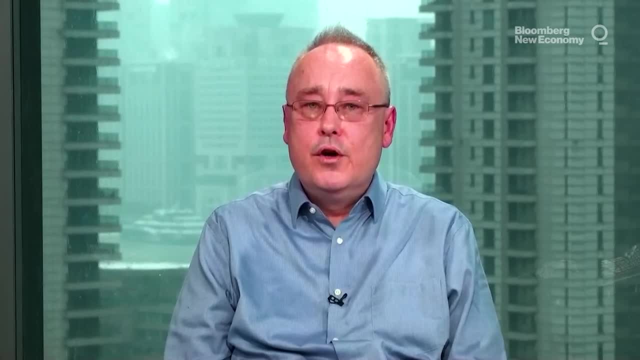 What is China's next strategy? And so this is the central challenge, because, as your economy grows, and even as you add all of this renewable capacity, you still need to make sure that the coal supply is flowing in order to keep the lights on. 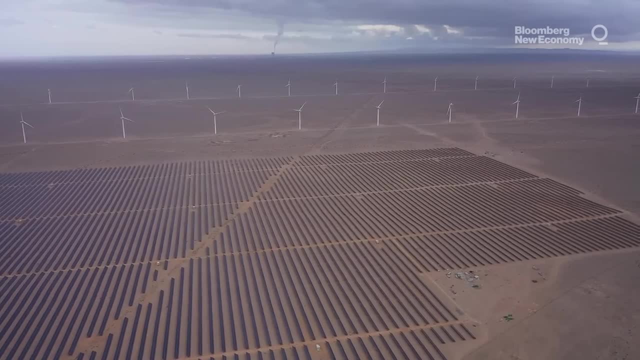 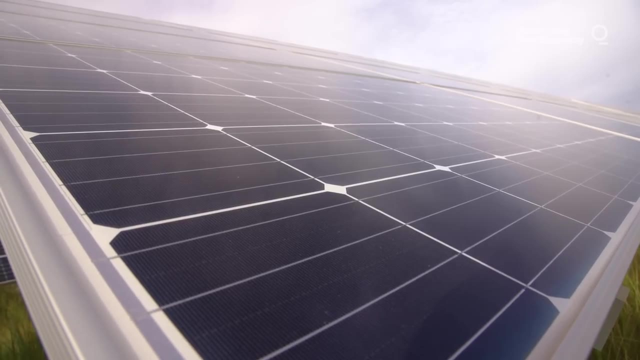 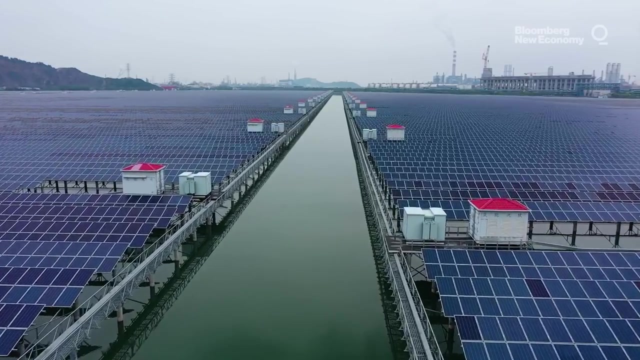 That's going to be the big challenge for policymakers. Even China's world-leading investments in carbon-free energy may not get them to their targets on time, But Beijing has recognised that the economic, political and environmental rationales for clean energy now vastly outweigh the costs. 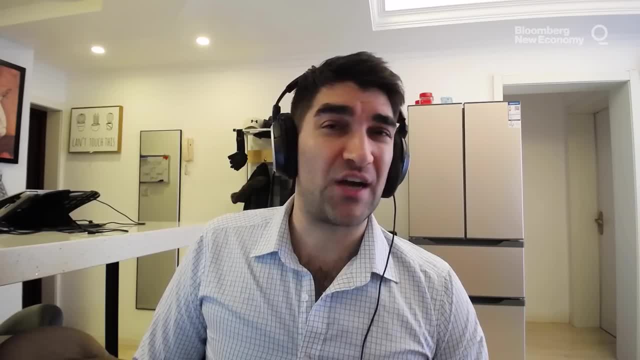 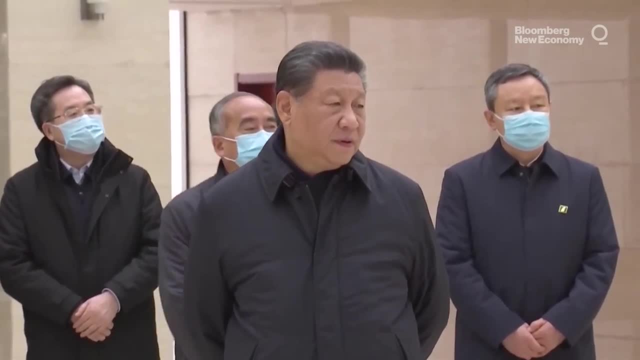 When it comes to the 2060 neutrality target, obviously China's a long way off and it's a huge, huge, audacious target. The people that are the top leaders that are planning it out right now they probably won't even be around to see it right.